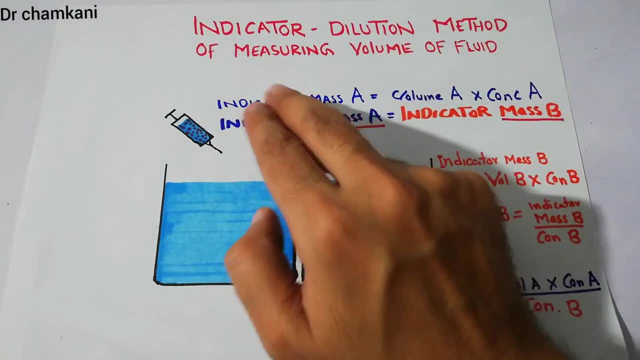 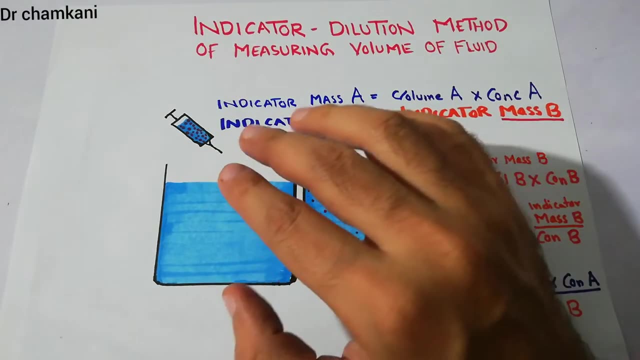 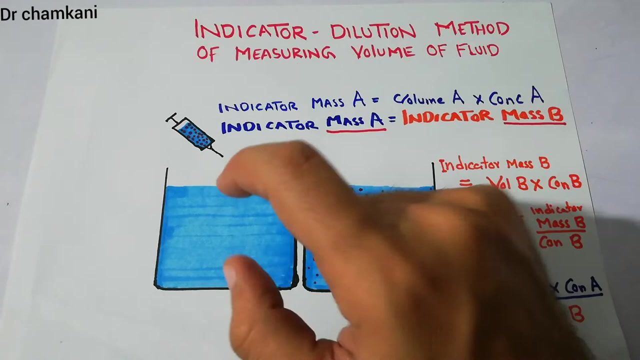 and the product of its volume and its concentration is basically its mass. Now there is law of conservation of mass and it states that the mass of this fluid, the mass of this fluid or the mass of this indicator, will remain the same. will remain the same after being put into another fluid? if no, 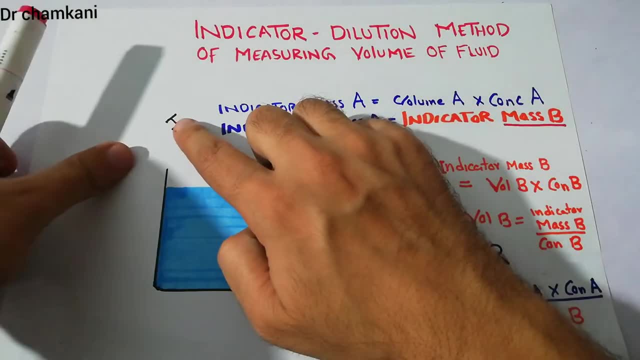 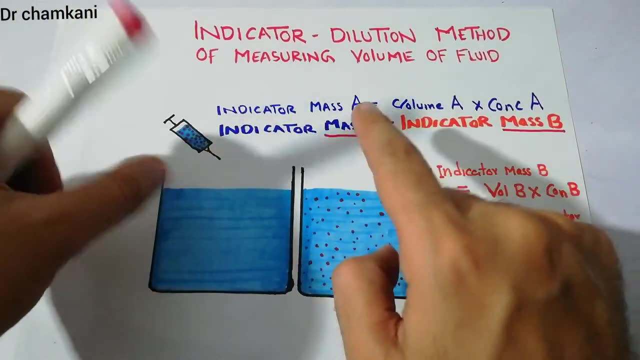 fluid is lost or there is no loss, Suppose, for example, while injecting this indicator into this fluid, while injecting this indicator into this fluid, if there is no loss of this fluid, then the mass here, the mass of this fluid, will be equal to its mass in this container. Now we call it mass. 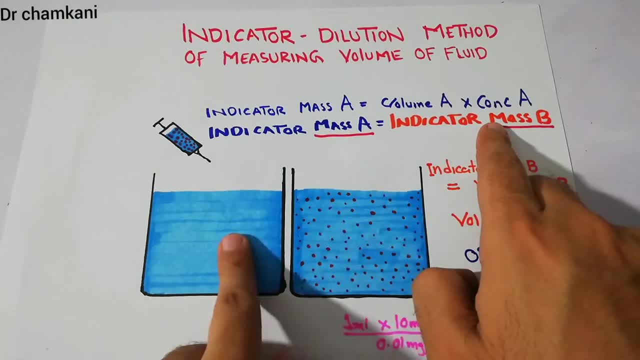 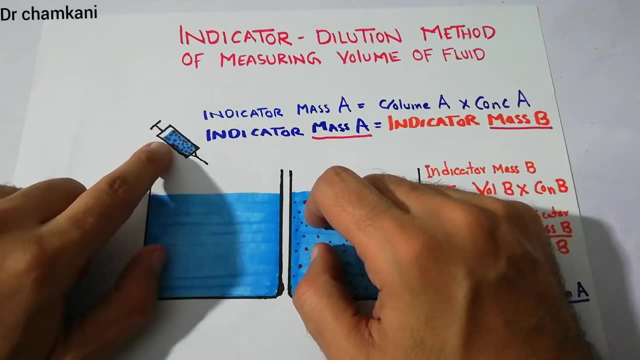 a when it is not injected, and we call it mass b when it is injected into this fluid, for example here. But there is one important thing and that is about the concentration. Here this indicator or this dye is very much concentrated. Its concentration is very much high, but when it 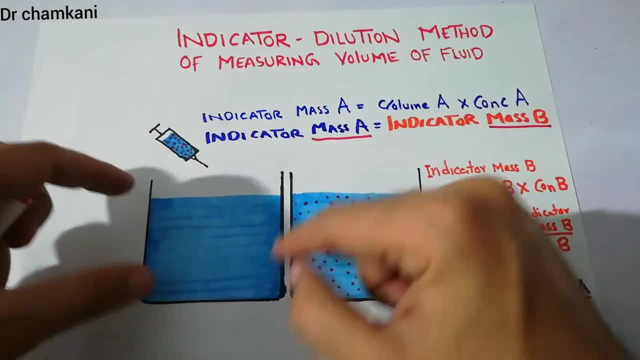 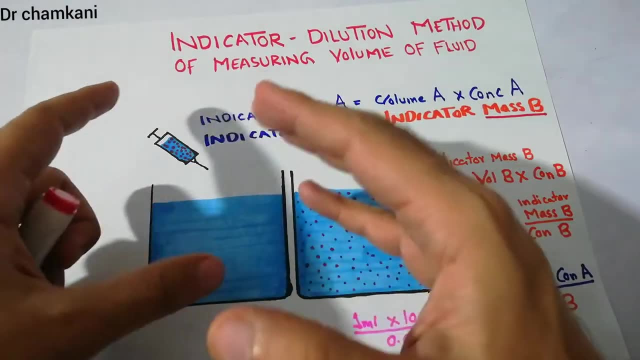 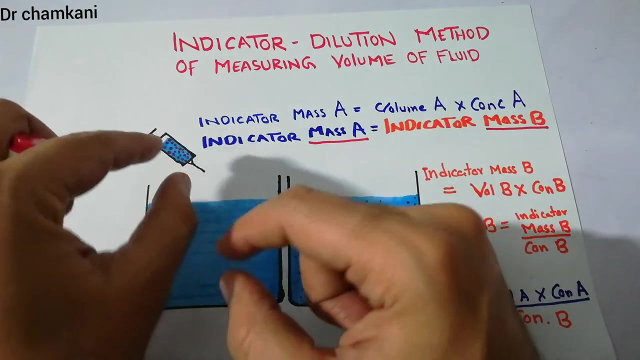 is put into a large fluid, or with when it is put into this large fluid, then this, this indicator, will basically dissolve and it will basically disperse in this fluid. so definitely its concentration is going to decrease or change. its concentration will change because because here this fluid or this indicator was present in small area in this, much but the same. 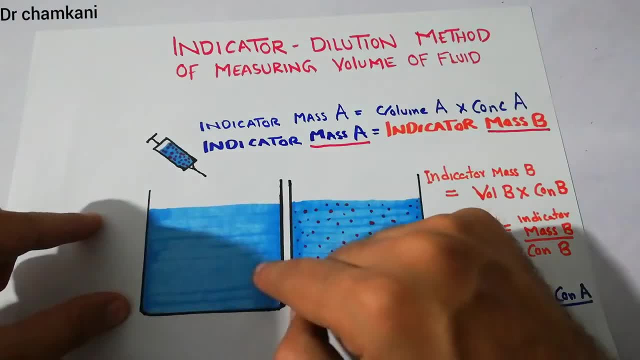 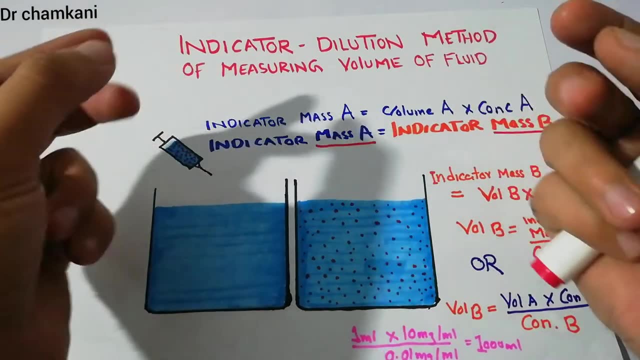 indicator. the same indicator has to basically distribute into a large area, so basically its concentration decreases. is, for example, this is one spoon of sugar and it is present in a few sips of water, then that that water, few sips of water, for example, in half the glass that will be. 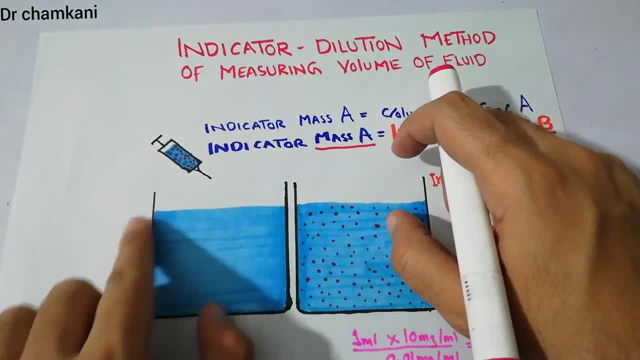 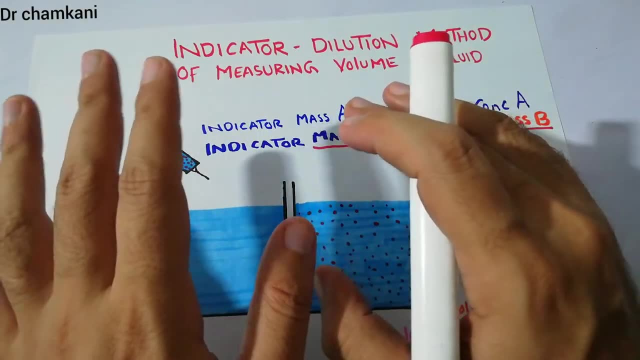 very, very sweet. but if we put that sweet water into four or five glasses of water, then that four, five glasses of water in a large container can container will not be that much sweet because the concentration will decrease, but but the amount of fluid remains the same and its mass. 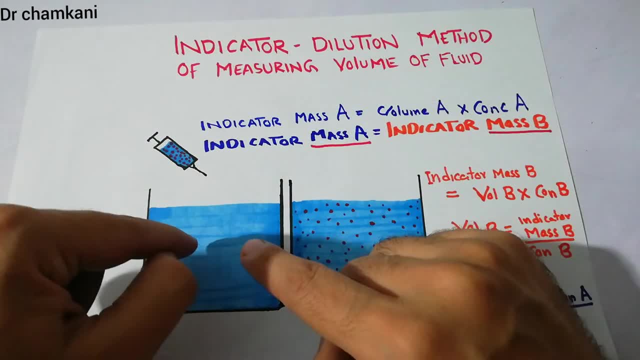 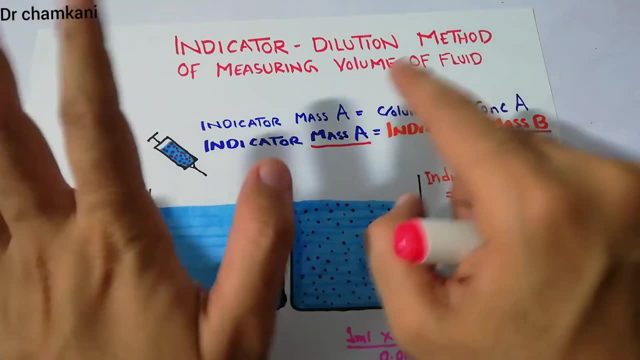 before putting it into this container is equal to after putting it into this container. but that is a simple difference. that is a subtle difference which we have to differentiate because it is going to be helpful. so before starting the experiment, the mass of this indicator is mass a and which. 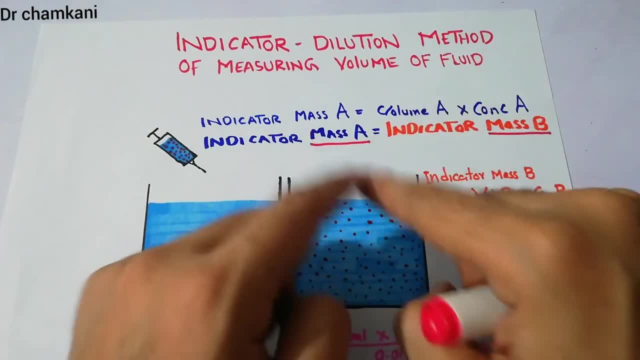 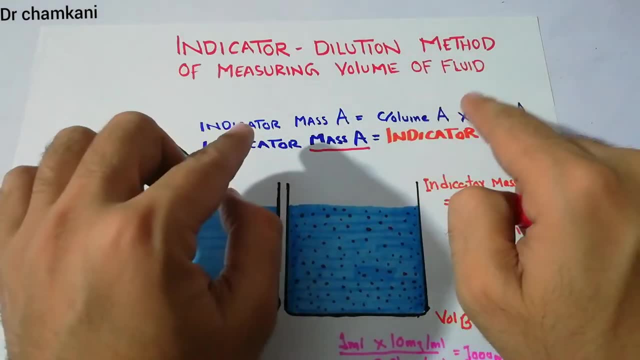 is basically the product of volume and concentration of this indicator. after being put into this container, the mass of this indicator is mass a and which is basically the product of volume and concentration of this indicator. after being put into this large fluid, it basically distributes and we call it is mass b here, indicator mass b, and we can say: due to the law of 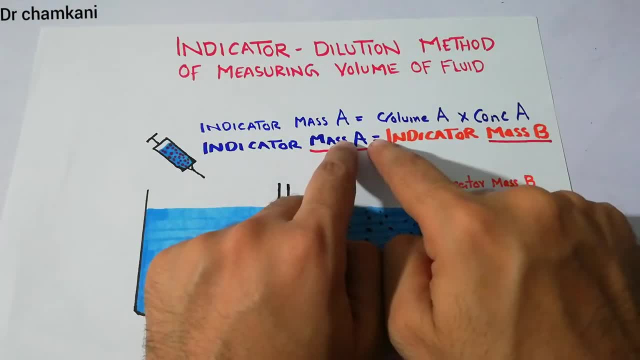 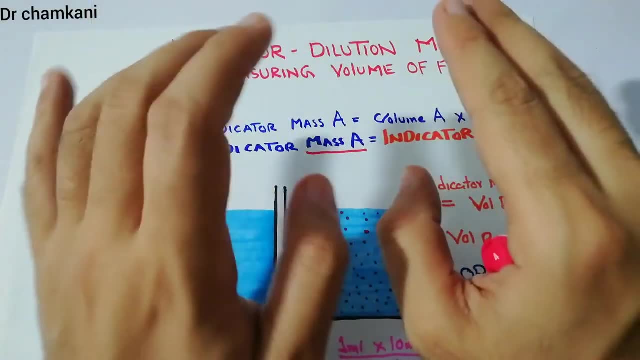 conservation of mass, that the mass indicator mass a is equal to indicator mass b, because this is the same thing, present here or here, its mass remains the same it, if there is no loss, if there is no loss of fluid, if there is no loss of fluid, its mass remains the same, here and here, its concentrations. 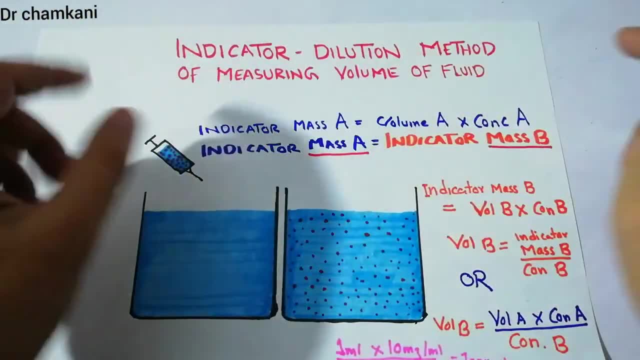 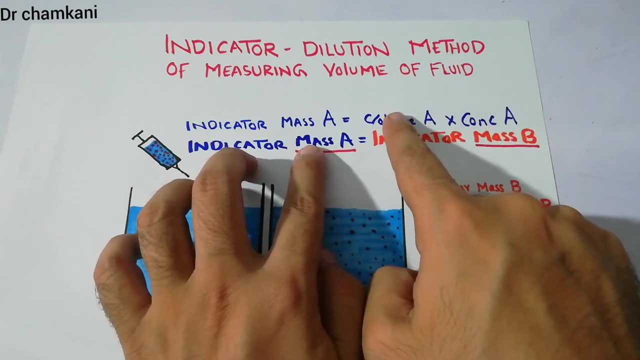 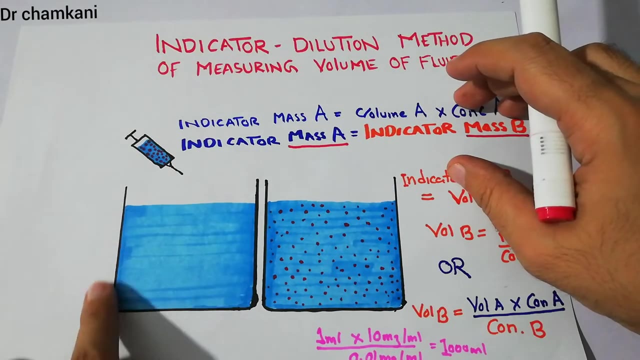 changes, its sweetness distributes, for example- but its amount remains the same. so the indicator mass a is basically equal to indicator mass b, and mass is always the product of volume into concentration. now what we do? that once this indicator has been put into this fluid. now we want to determine the volume. 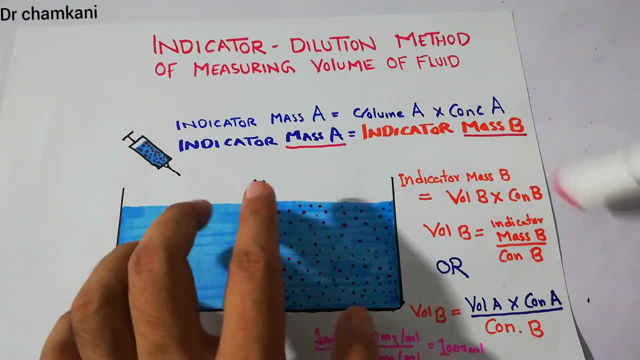 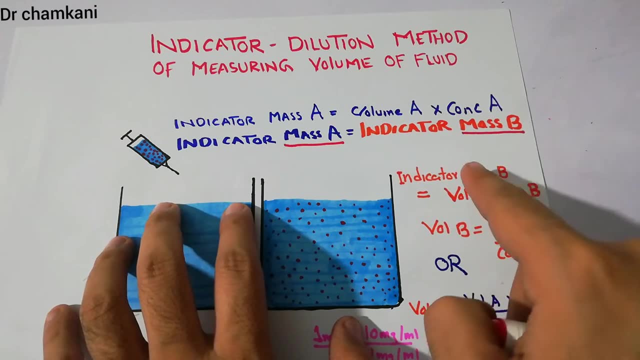 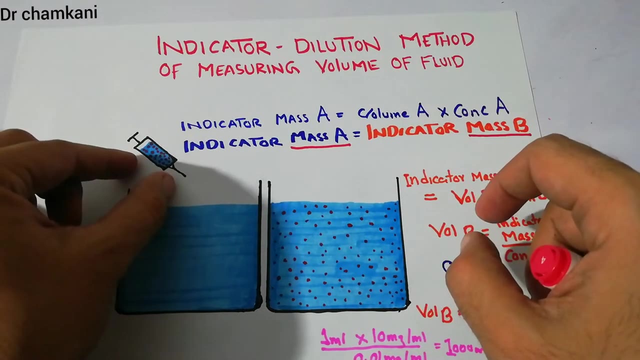 of this fluid. we want to determine the volume of this fluid. so when we put it here we can say that the indicator mass b is now equal to the volume b into the concentration b, or the mass b is basically the product of volume b in concentration b. but try to remember that it is the same indicator, only its 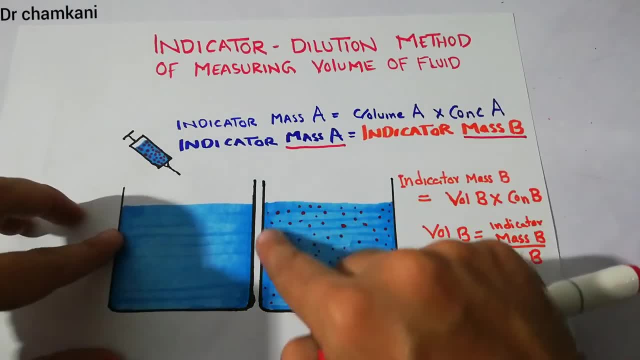 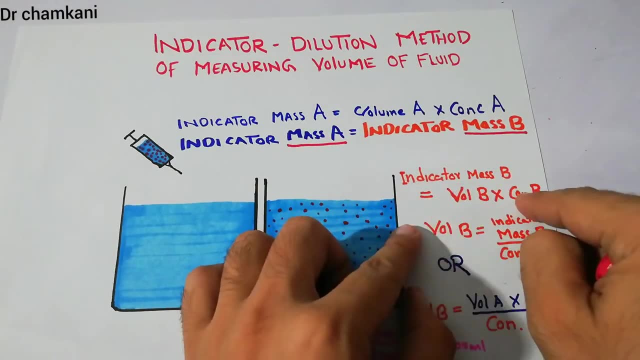 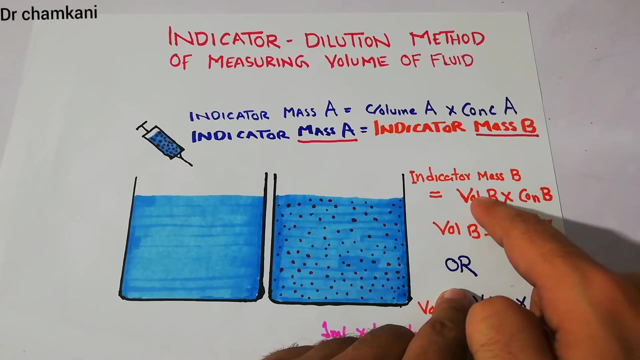 concentration has changed. only its concentration has changed because it has distributed over a large area or in a large fluid. now, mathematically we know that we can shuffle this equation. mass is basically equal to product of volume into concentration. mass is equal to volume into concentration. so volume is basically mass by concentration. volume is mass by concentration. 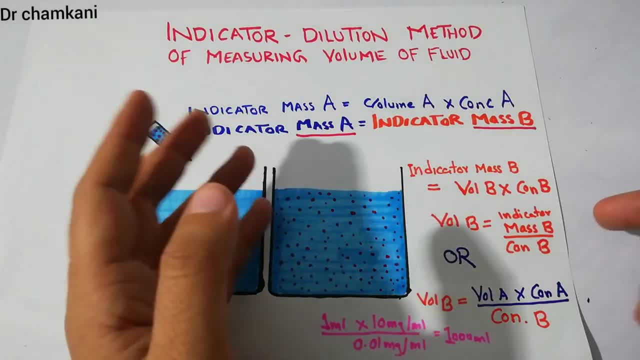 this is basically the shall shuffling of this equation, which is basically a mathematical rule that once you know two things, we can determine. basically, the two categories of concentration are allowed to be realized by the calculation. you need to know the degraded mass count, emmar. we are 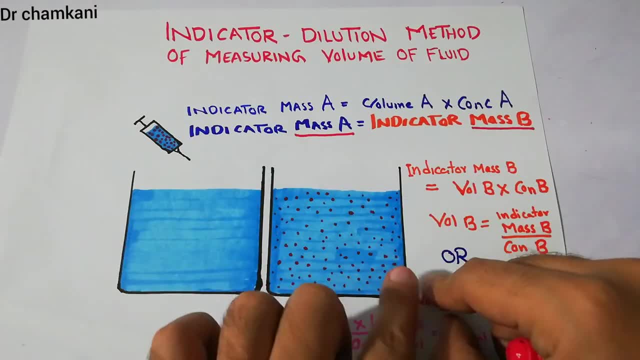 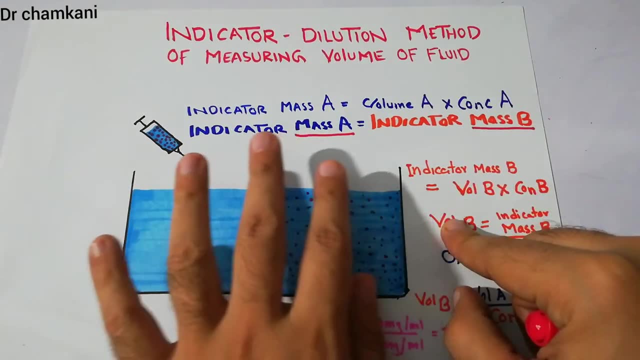 third thing: so we are basically more interested in its volume. we are basically more interested in its volume. now this, uh, this fluid is. now we are going to determine the volume of this fluid, but its concentration has changed. the indicator present, the indicator that we put in this fluid, 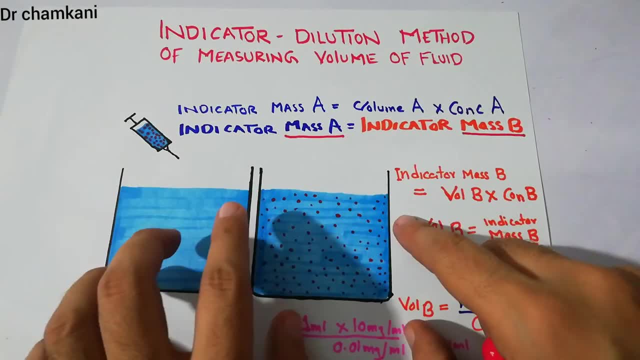 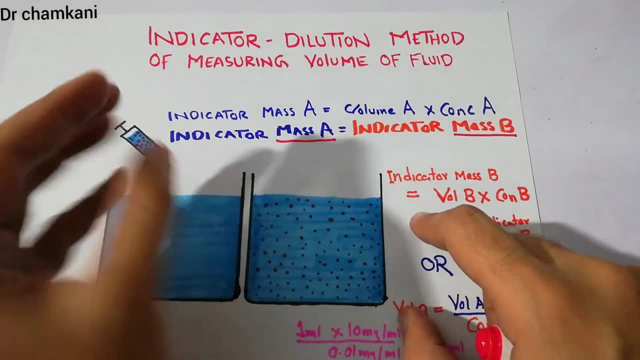 remains the same. its volume remains the same. but we are more interested in the volume of this fluid, because we know the volume of this fluid. its mass remains the same. its mass, the amount in this fluid, remains the same, but its concentration, it basically disperses over large area. so we need 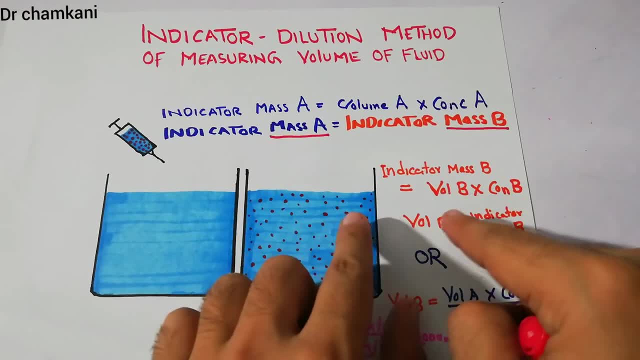 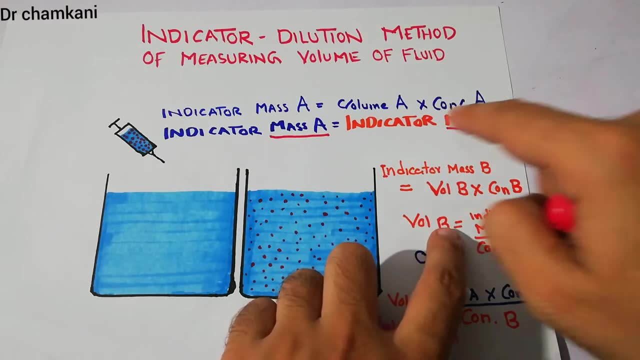 its volume now or its large area. we need its volume now. so basically we need the volume for the volume. this equation basically becomes mass by concentration, mass by concentration. from this equation here, from the law of conservation of mass, we know that the indicator b, mass, is basically. 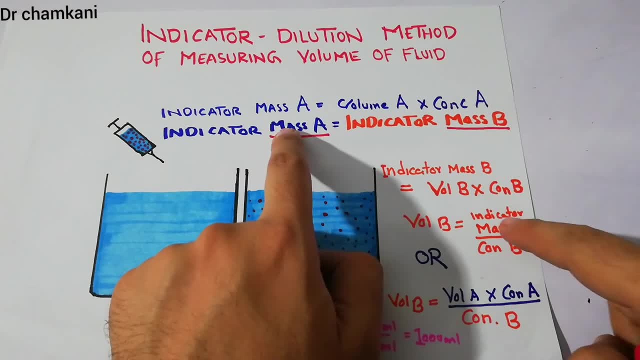 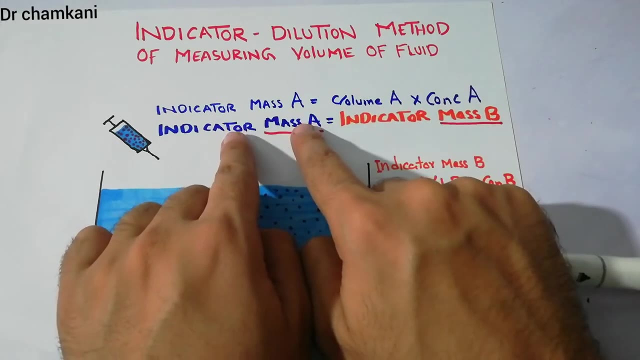 equal to mass a. mass b is equal to mass a, so we can also write mass a instead of mass b. mass b is equal to mass a, and here we have the mass b where? here we have the mass b. so instead of mass b we can write the mass a, because they are equal. mass a is equal to mass b due to the law of 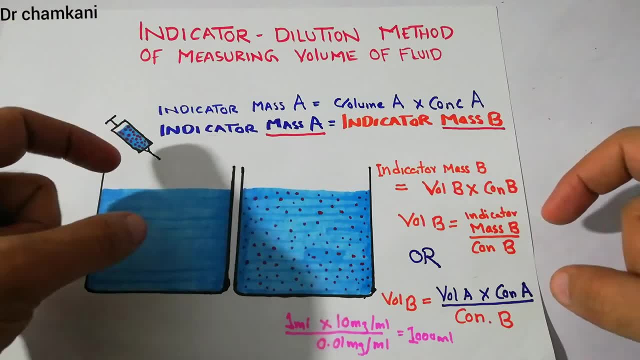 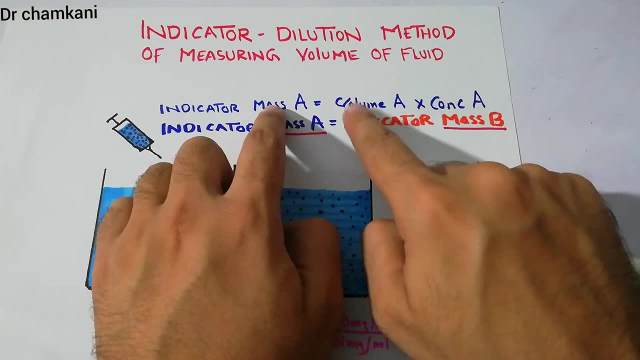 conservation of mass. now we are doing these changes just to determine the volume, because here we don't know the mass of this fluid. but if we look at it, we know the volume of fluid mass. we know the volume of this fluid and we also know the concentration of this fluid. so instead of 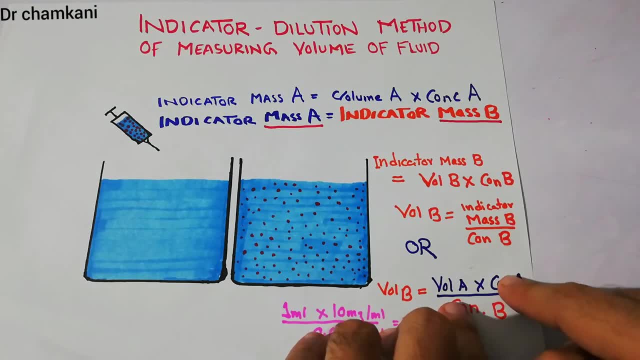 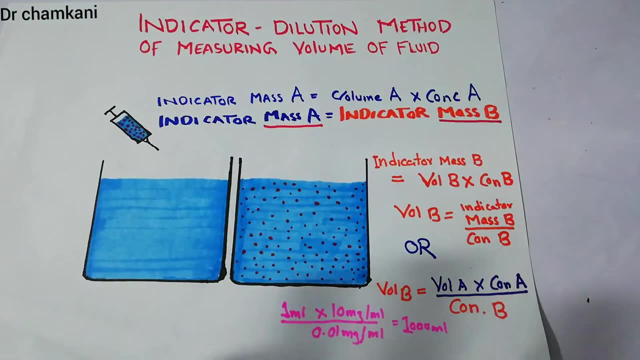 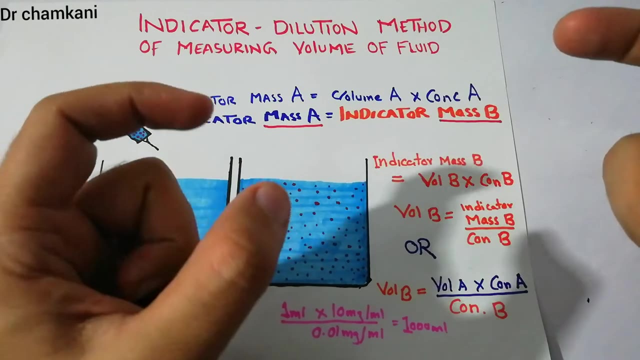 writing this mass b. we write mass b, volume a and concentration a because mass b is equal to mass a and then mass a is the product of volume a into concentration a. we just, you just need to focus on it. this is basically a mathematical equation. it is uh mathematical and uh, if you focus, you will come to know that it's. 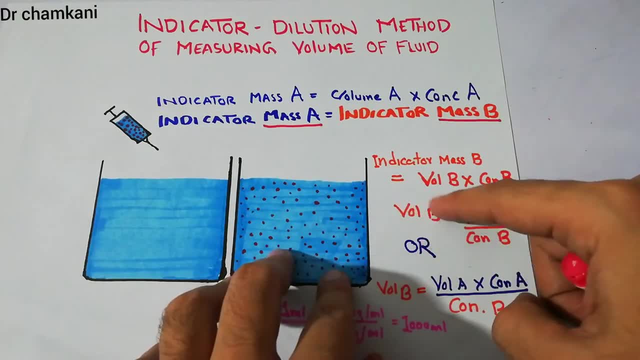 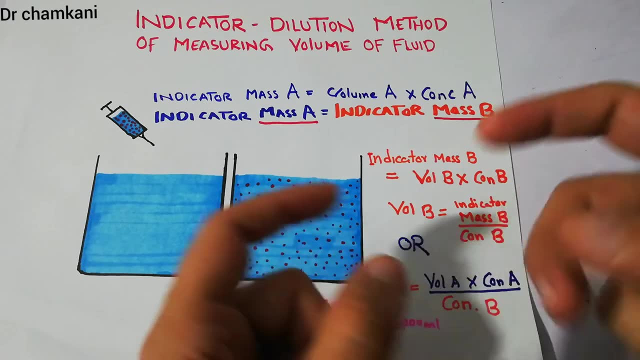 very simple as well now. the the purpose is to determine this thing, determine. the purpose is to determine volume and to determine the volume. we basically need all those values which we know now. we don't know the volume, but we know the volume of the fluid and we know the concentration of. 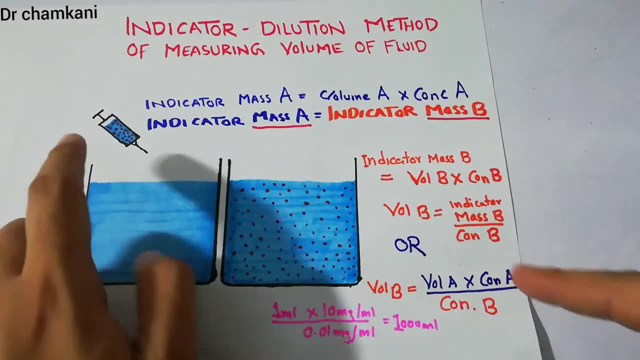 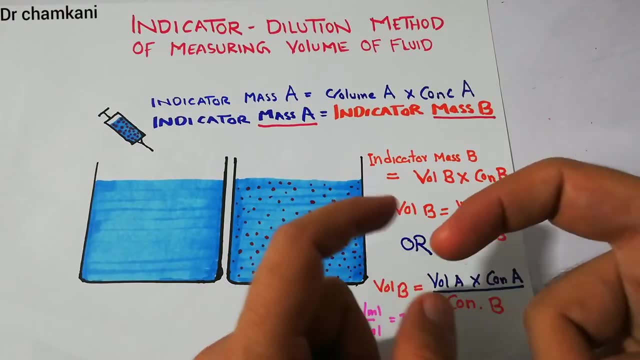 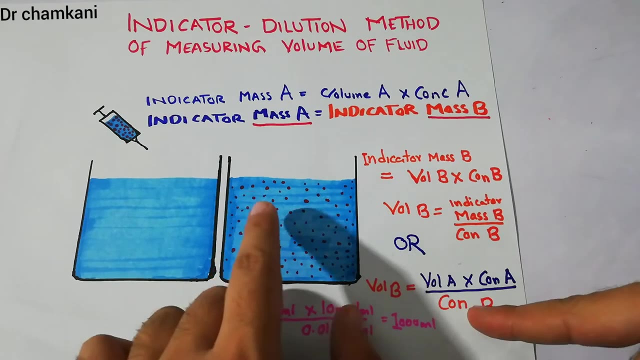 this indicator, we know the concentration of this indicator and we can basically determine the concentration of this um fluid with some uh, a machine or through any way. we can determine its concentration and we also know its concentration of this indicator. so when we determine its concentration and we also know the uh, the volume, and we also know the concentration, we put those. 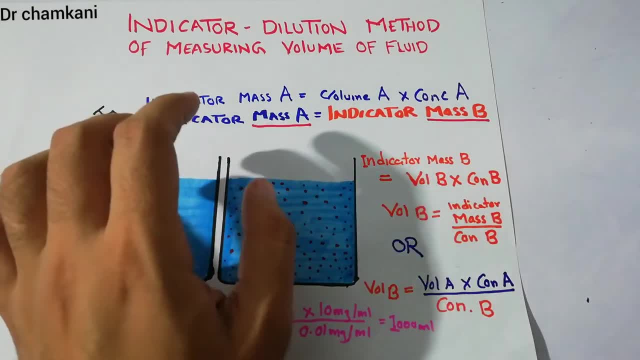 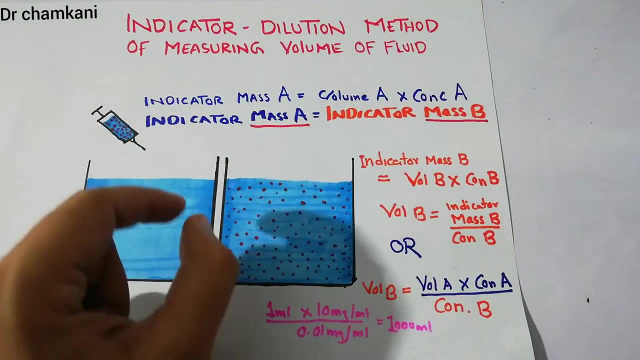 values and we can determine the volume of this fluid. so there is simple rule, and that is the law of conservation of mass, that the mass of this fluid, before putting it and after putting it, remains the same. so mass of a is equal to mass b, and this is the same fluid, but but its volume. 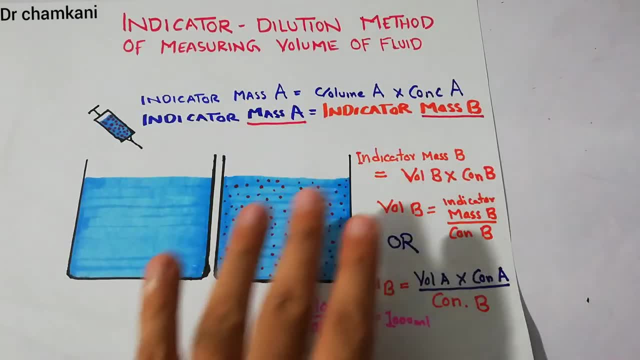 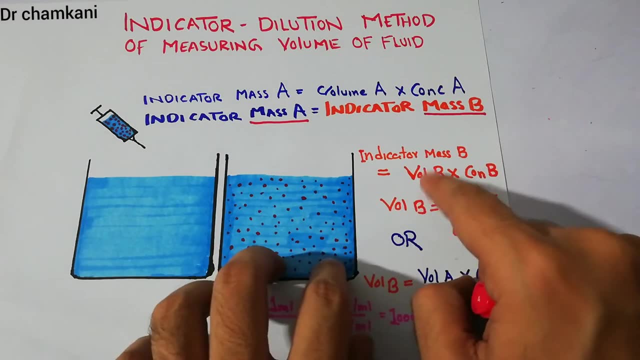 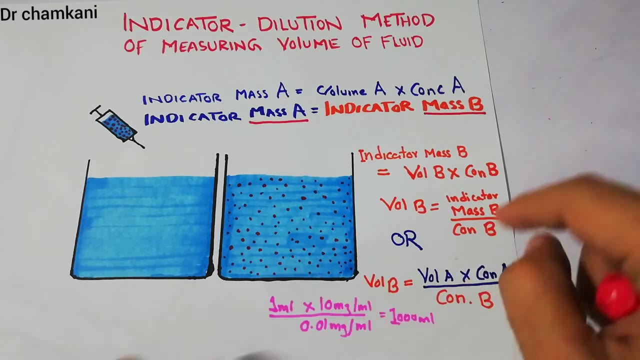 basically changes and it it distributes over a larger area, so its concentration changes. now we basically shuffle this experiment. sorry, we shuffle this equation and we basically want to determine the volume b. so to determine the volume b, we put those values in this equation and we can determine the volume b. now suppose, for example, with this experiment, with these values, it 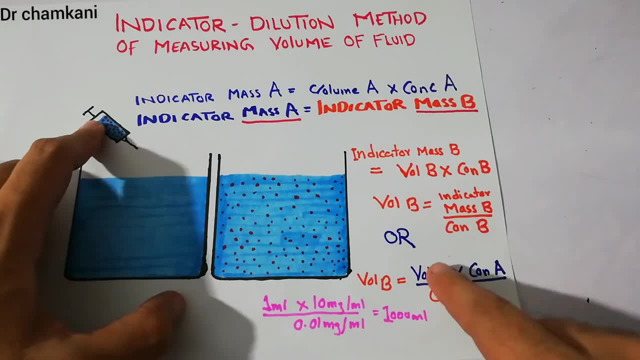 will get clear that suppose, for example, the amount or the volume of this fluid was one ml. we knew that the volume is one ml, so we put that value here in this equation. we put that value one ml instead of volume a. now we also knew the, the concentration of this fluid, and that was around. 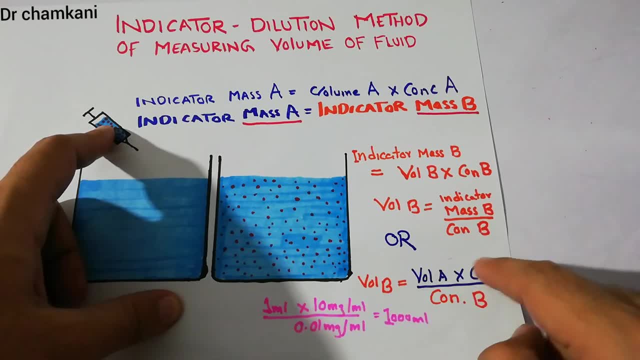 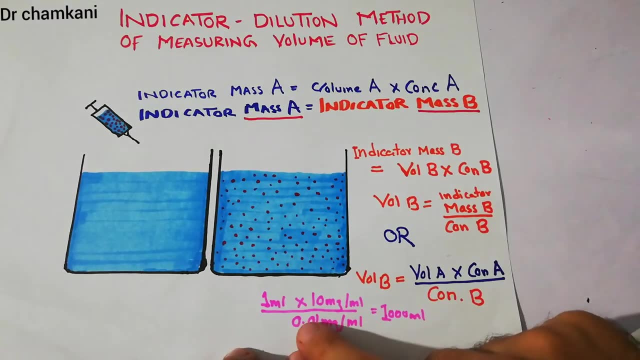 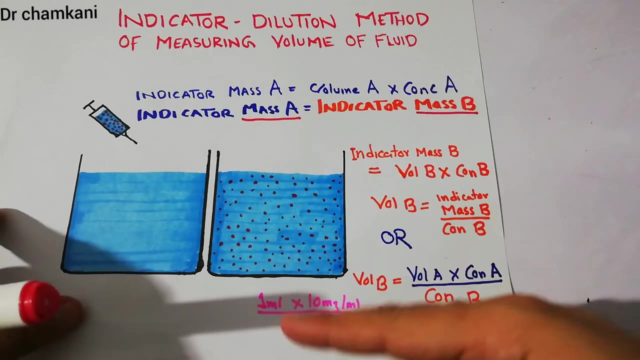 10 milligram per ml. so we put that concentration here in this, this equation, one into ten, and after putting this indicator into this fluid, its concentration became zero point zero one. now, this zero point zero one has been determined. this has been determined through some machine or some uh experiment, something. now, this has been determined. and when we put 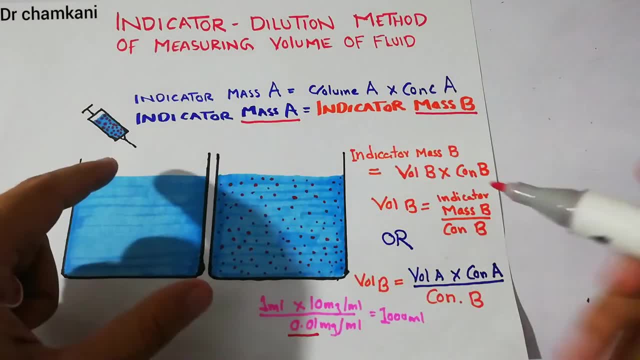 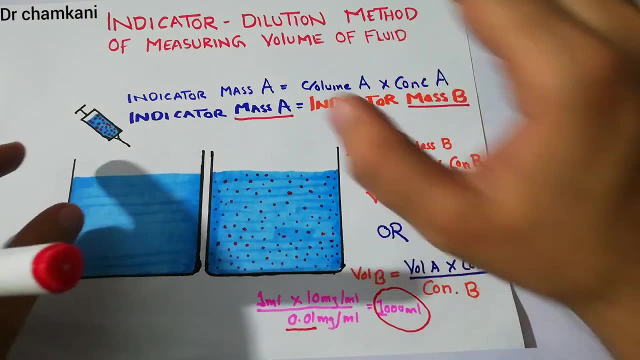 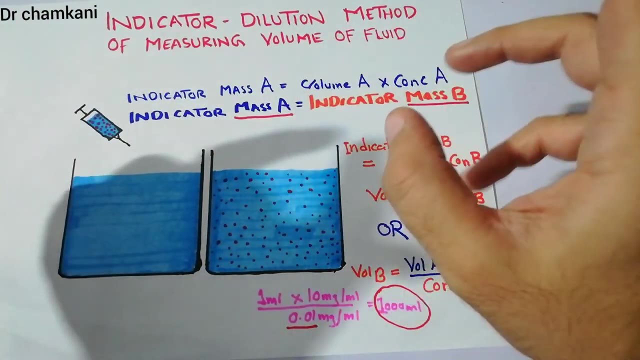 that concentration in the equation, we get the volume of fluid b, we get the volume of fluid b. so this experiment or this method simply means that we put an indicator and it gets diluted. so it is the indicator dilution method and we uh, through law of conservation of mass. 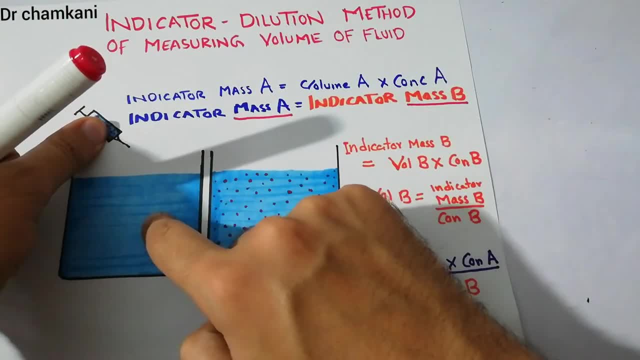 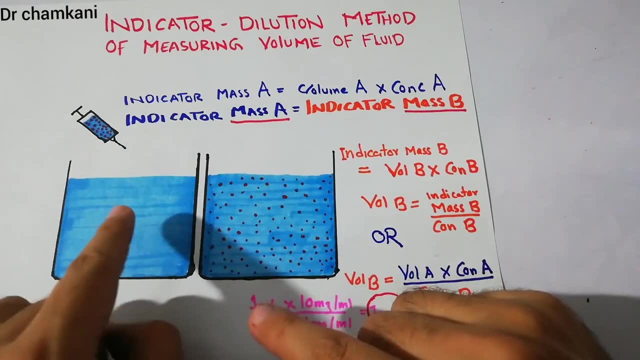 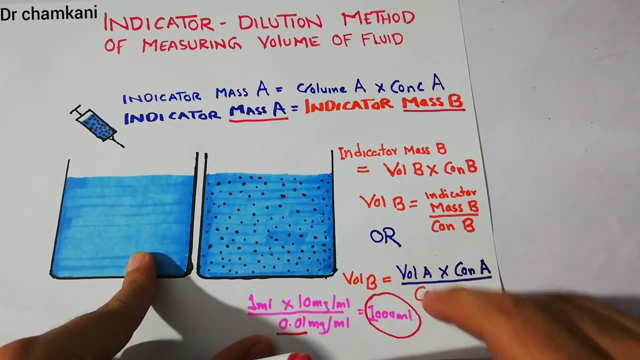 we know that the its mass before putting it and after putting it remains the same. if it is one ml, it remains one ml before putting into this fluid and it remains one ml even after putting it into this fluid. but but its concentration changes. its concentration initially was 10 milligram per ml. 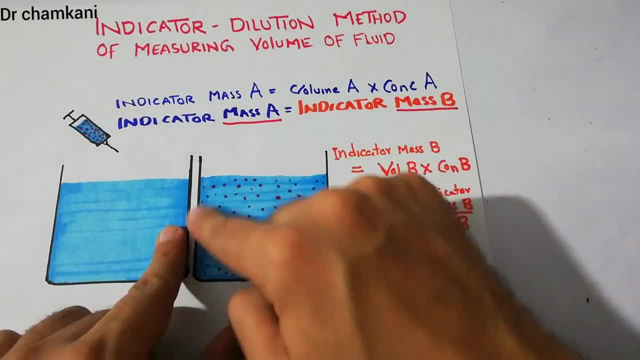 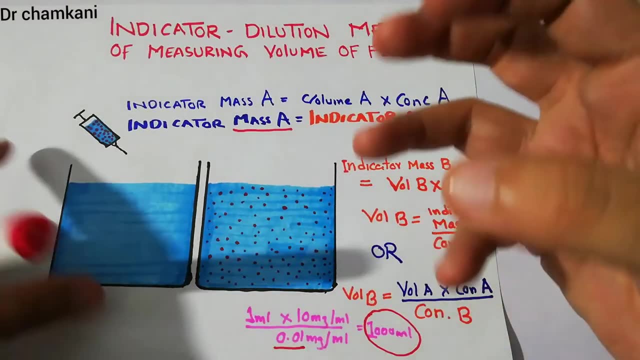 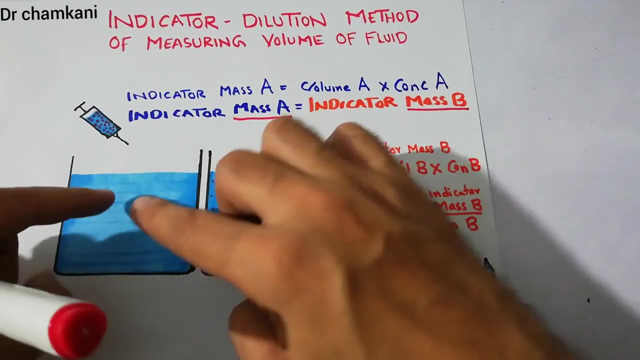 so the concentration of a was 10 milligram. when it gets distributed over this large fluid, its concentration decreased to 0.01, that is the concentration of b. so we determine that concentration through some machine or something like that experiment or any lab method, and then we, when we put those values in this equation, we can easily 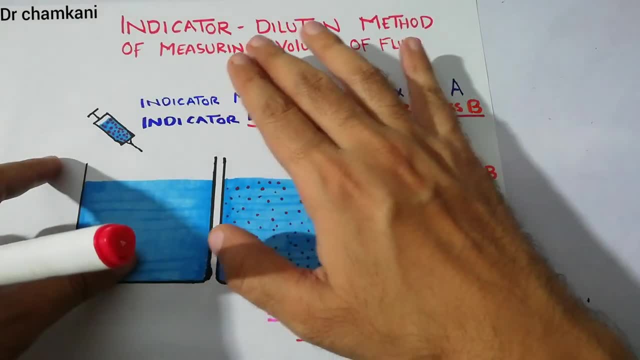 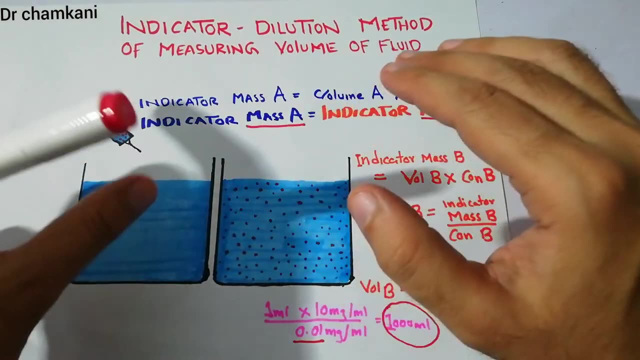 determine the, the volume of this fluid. that is basically the indicator dilution method for determining the volume of any fluid. now we are going to use this method, this indicator dilution method, and we are going to discuss that, how this method is basically used to determine the amount. 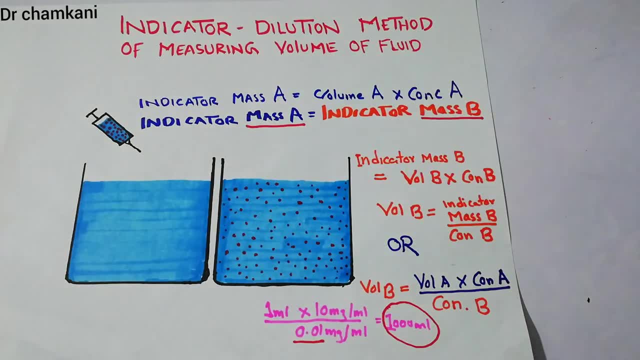 of fluid in the human body. now, that's all about the indicator dilution method. thanks a lot for watching the video.